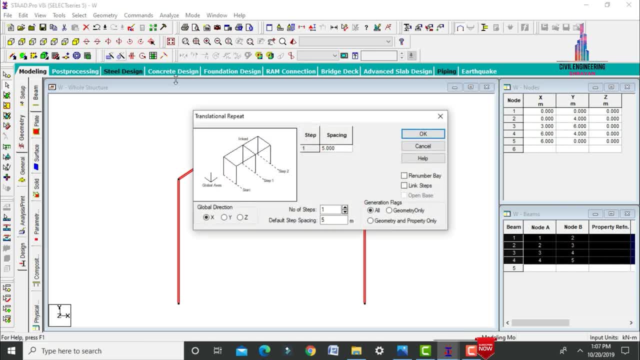 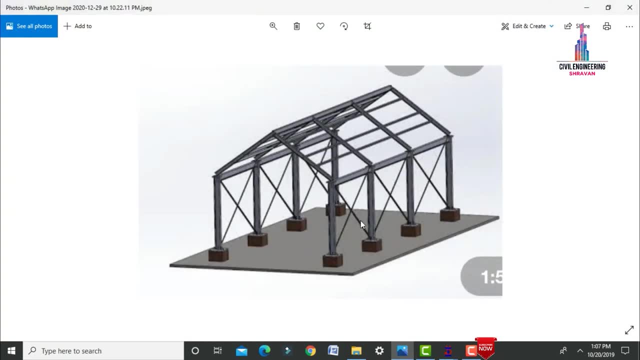 of this respected frames, by using control a option, Go to transitional repeat which is in z direction. So here we have to assume this respected spacing options. So, as per this respected figure, we are assumed that number of columns in this respected z direction are 4.. So it was created. 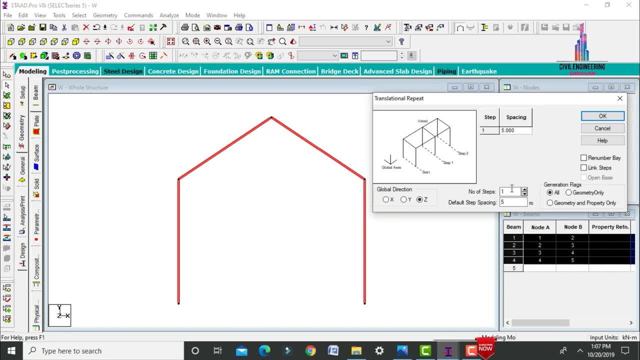 with one column here, So we have to copy remaining 3 columns. So for that initially we have to take, the number of steps are 3 and each step will be consisting of 4 meter. Click on link steps option. Click on ok. 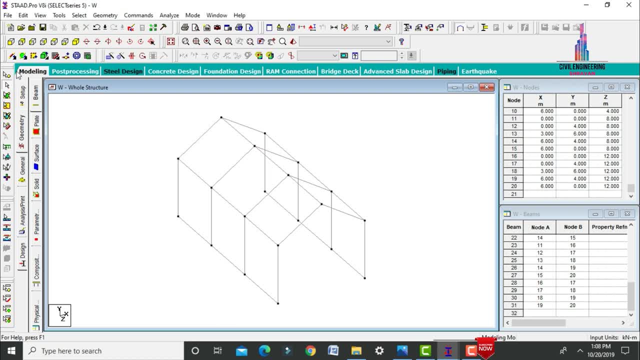 now we can see the warehouse model was created here like this. so after that, select the front view option. select all the beam sections at the base. so click on delete option. click on as well. so after that we had to add the bracings for this respected warehouse. so for that, select. 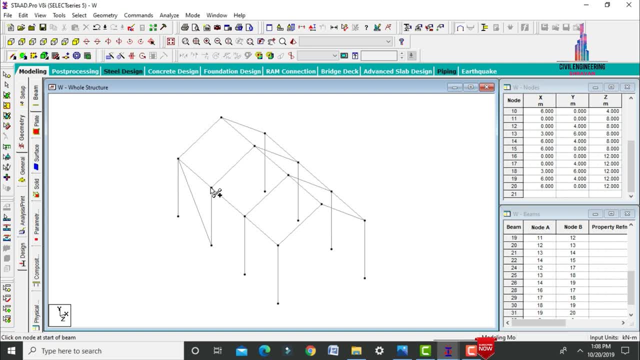 add beam command here: select the first point, select the second point, select the first point, select the second point. in the same way we had to add the bracings for the respected whole model. so here i'm rotating the model. here again we have to add the bracings for the right hand side also. 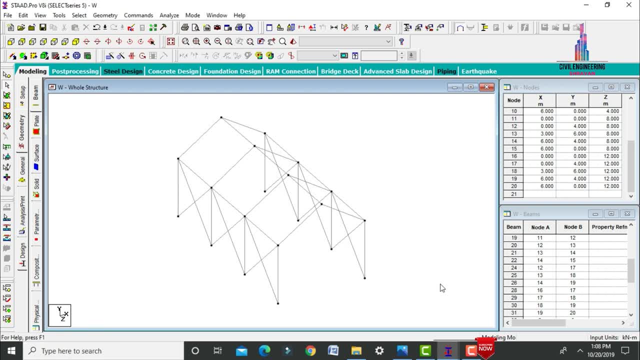 so after that, click on 3d model. so after adding the bracing sections, we have to add the members, which is supported on the top of the row. so for that, initially we have to select the top view, so we have to select all the beam sections here. so here i'm selecting all the beams like this: 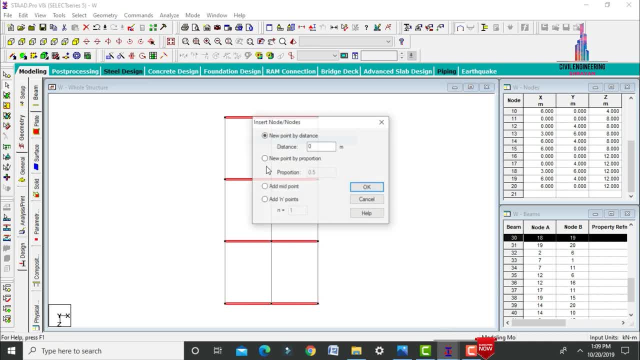 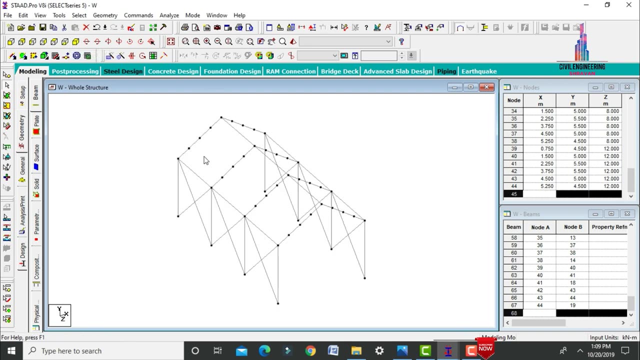 so click on insert node. so here i'm taking number. of nodes will be consisting of three points. we will check this in future. click on ok so it will insert this respective node points here like this: so after that, click on this respective 3d model. so it was created, your respective node point with equal distance. 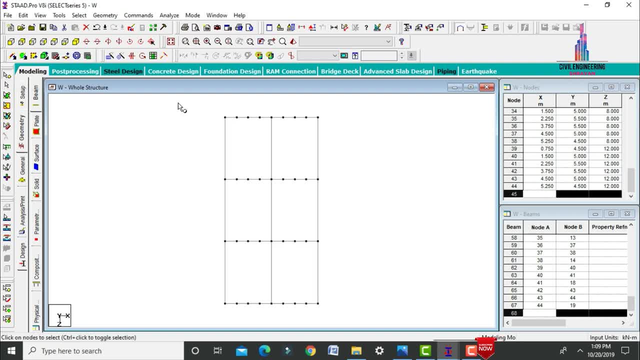 ok, so after that select top view. so here we have to select the node cursor. just, i am selecting the nodes for this respective right hand side section. again i am selecting the nodes for this respective left hand side section. so click on 3d view. so we have to connect this. 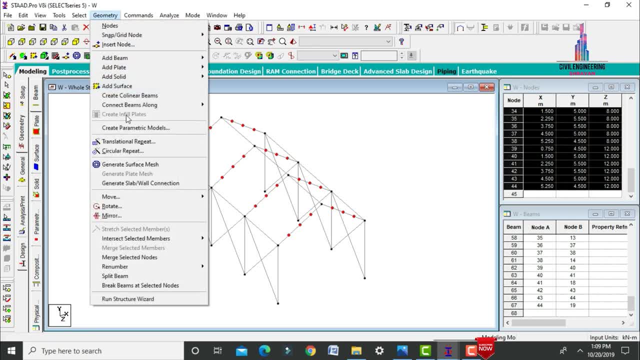 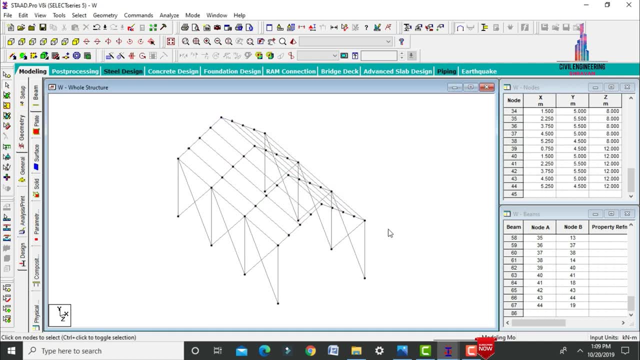 respective node points with the help of the beams. so go to geometry, connect the beams along z axis, so it will create 80 number of the beams for this respective warehouse section like this. now we have to see this respective whole model in rendering view, so click on. 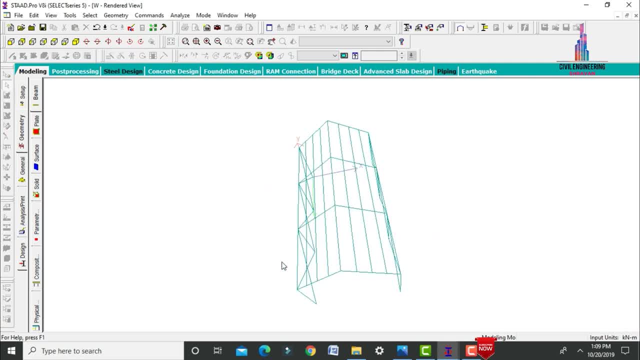 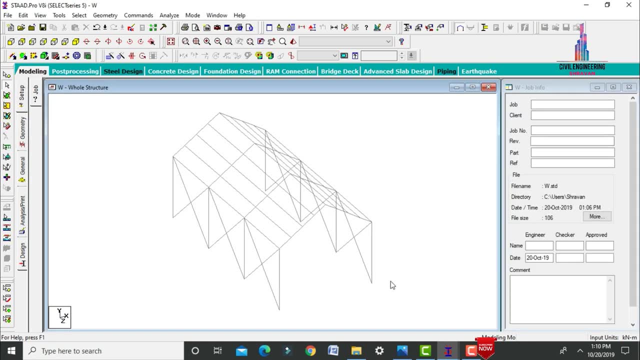 rendering view option. so this is the rendering view for this respective lines- nothing but your grids for this respective warehouse. so after modeling process completed, we have to assign the beam sizes and column sizes and this respective member sizes for this respective warehouse. so for that, initially we have to create the steel structure models from the 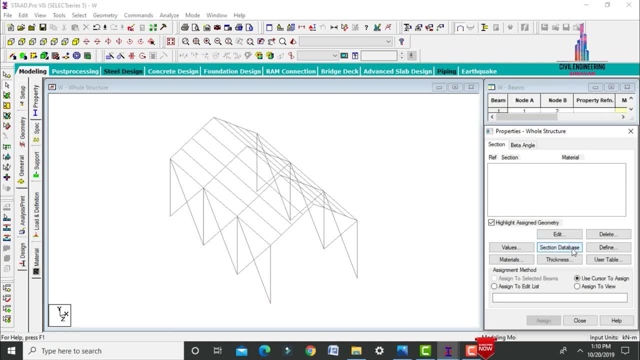 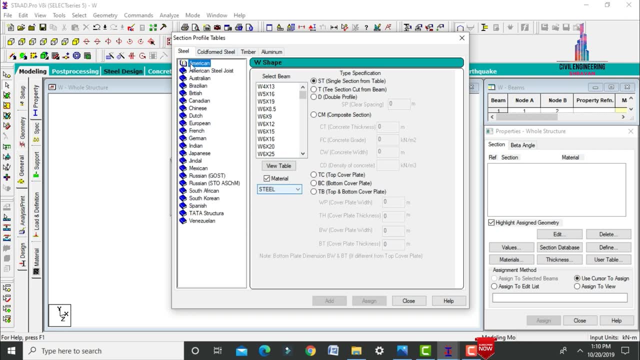 database. so for that, select general option here, click on section database so it will open this respective section database values like this. so in this we have to select as per the indian standard system. just i am selecting, so here i am selecting double section. so we have to select any one of the section from this respective model. so here i am considering. 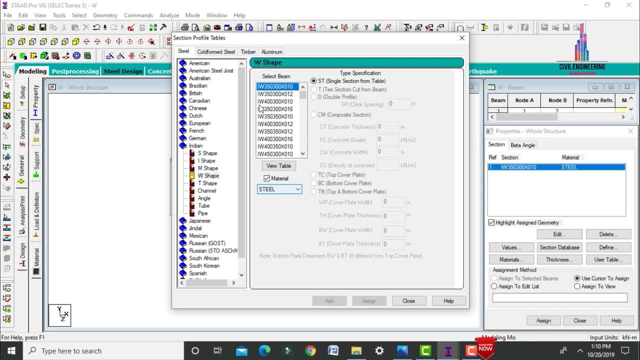 350 by 300 by 10, model 1. ok, so here i am selecting 350 by 300 by 10, model 1. ok, so here i am selecting 350 by 300 by 10, model 1. so again i will take 350 by 300 by 12, model, another one: ok. so after that i will add angle. 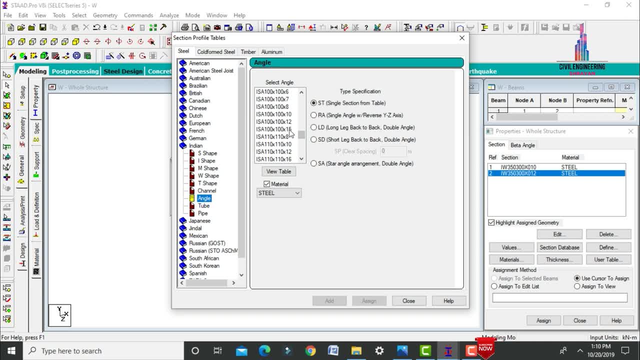 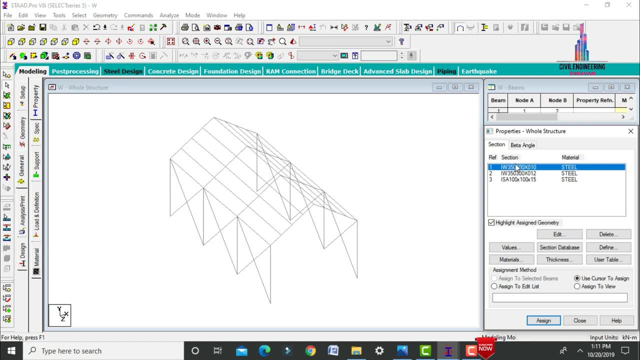 section so, which is consisting of, let us assume, 100 by 100 by 50. click on add button, close option. so here we have to select this: respected: 350, cross, 300, cross 10. we have to assign this respected, or we have to assign this respected property for the horizontal members. so here: 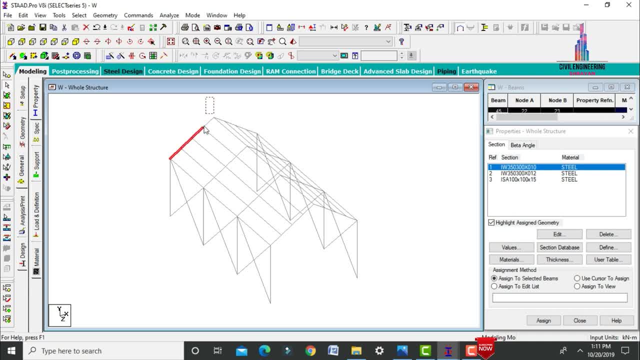 i am selecting horizontal beam sections for this respected warehouse like this. so after that, select this. respected vertical members also now here we have to select the right hand side members, also for this respected model. so here i am selecting this models. so after that, click on assign to selected beams. assign yes option. again we have to select. 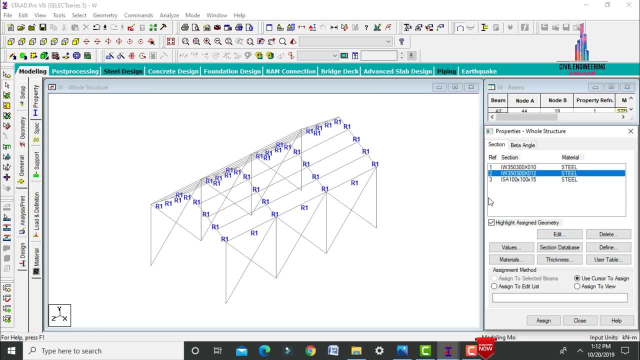 odd 2. just, i will assign this respected odd 2 for the column sections. go to select option: beams parallel to y-axis. click on assign to selected beams. assign yes option. so here i. So after that we have to assign this respected ISA 100x100x15 for the remaining models. 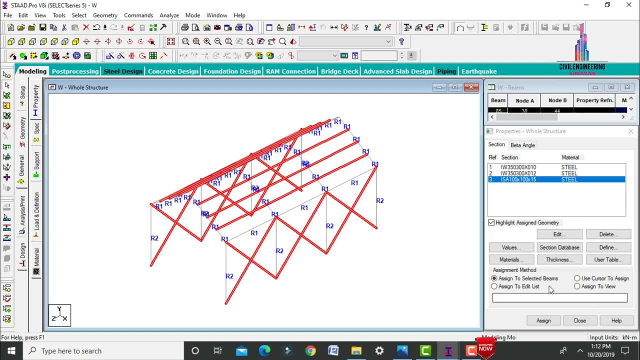 So go to select by missing attribute, missing property. click on assign to selected beams here. assign yes option. After assigning the properties, we need to see this respected whole model in rendering view. So click on 3D view. click on this respected modeling option. click on rendering view. 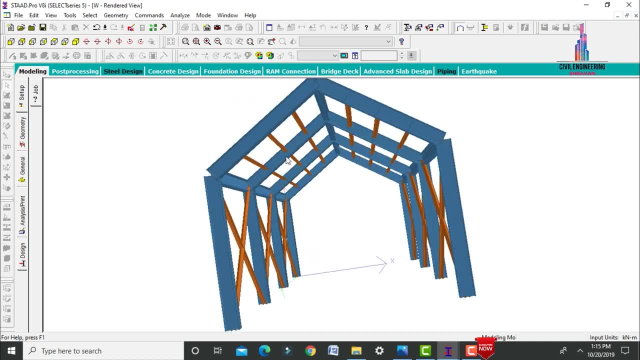 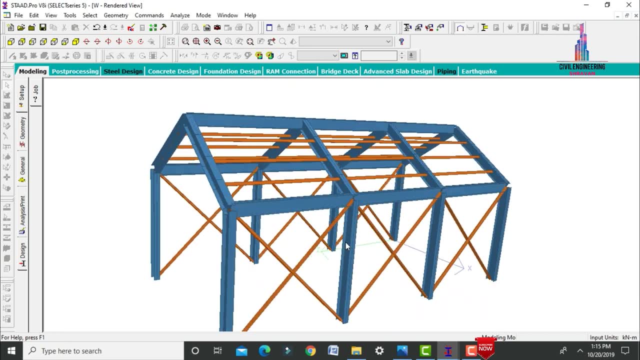 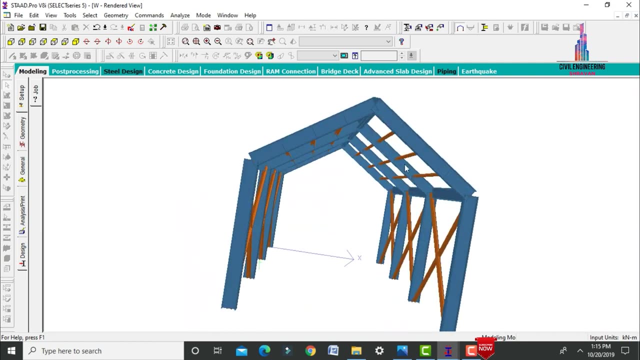 So this is the rendering view for this respected warehouse. It will be consisting of 350x300x12 is the column size And 350x300x10 is the beam sizes And the remaining sections. I will consider it as angle section, which is consisting of 100x100x15, okay. 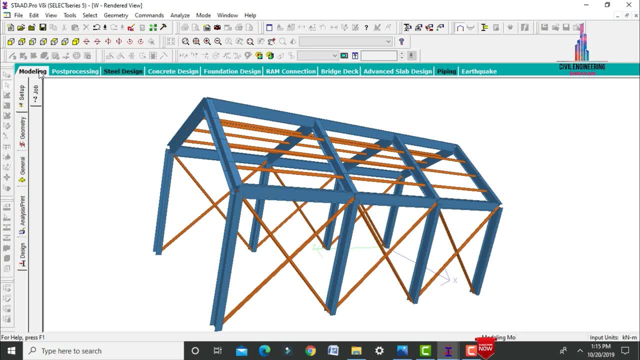 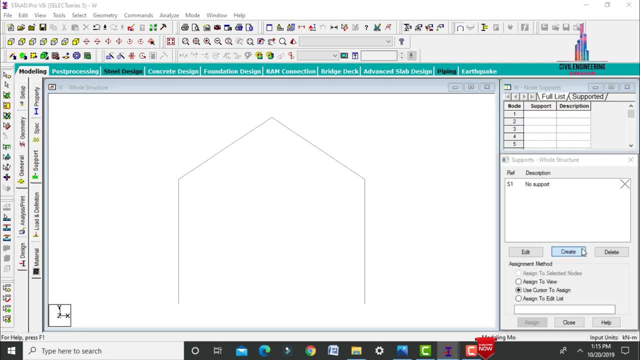 So this is the rendering view for this respected warehouse. So after that we have to assign the supports for this respected warehouse. So click on general option, select the supports. select the front view. So initially we will create the fixed supports. create option. click on add. select the support to select the node points. all the node points. 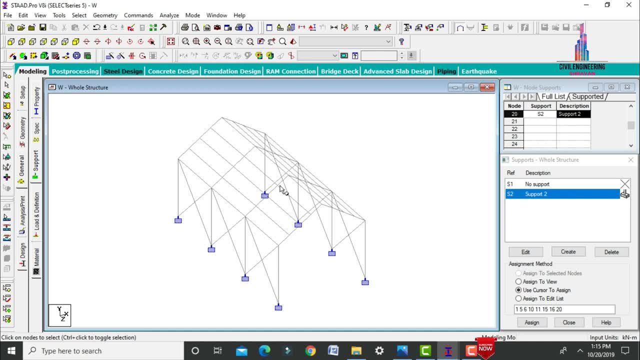 Click on assign to selected nodes. Assign: yes. So after that we have to define the load cases, which is related to the respected seismic loading condition. So as well as wind loading condition, But as per IS 875, part 3,, it was suggested that if the structure or any one of the building which is greater than your 10 meter, we need to apply the wind loading case. 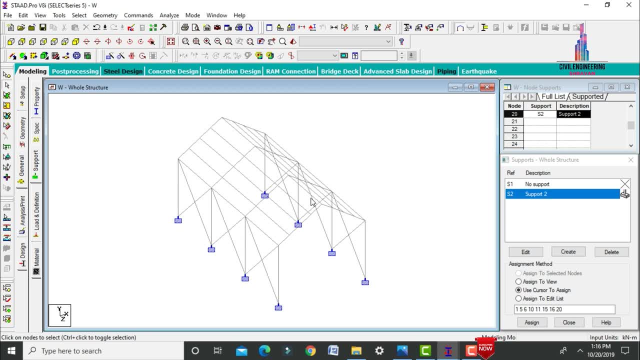 Otherwise we can skip the wind loading conditions. So for this respected warehouse, I was considered it as height as 6 meter. So that's why I am eliminating the wind loading conditions. okay. So for this respected warehouse, I was considered it as height as 6 meter. 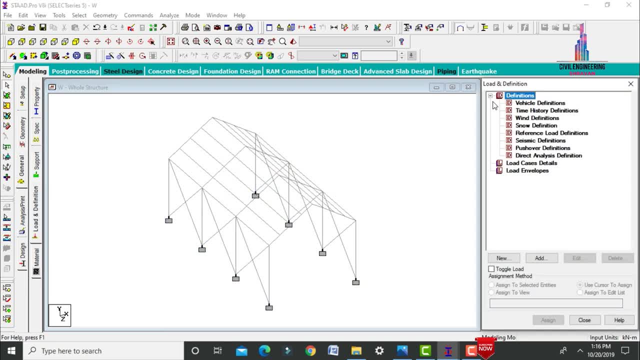 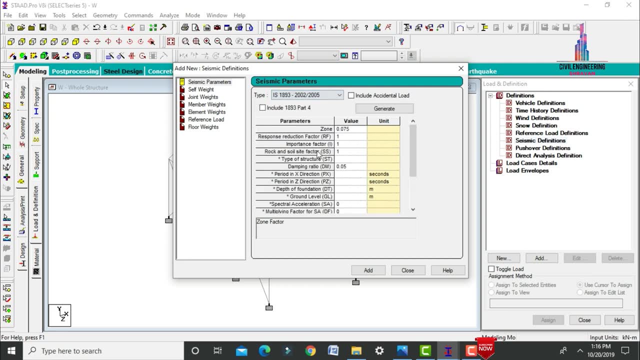 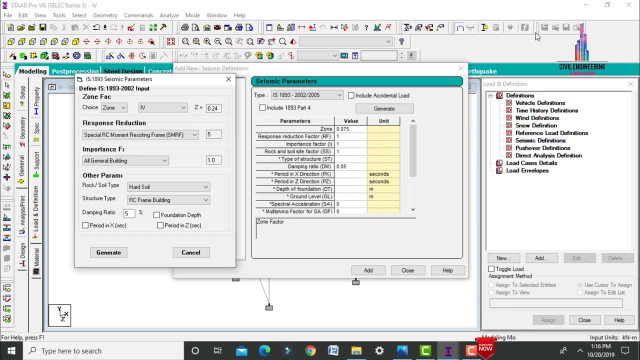 So for that, initially we have to define the seismic loading condition. Select definition option. select the seismic definitions. click on add button. So here we have to select the IS code- IS 1893, click on generate option. So here I am, selecting the zone which is consisting of zone 4, which is having the factor of 0.24 condition. 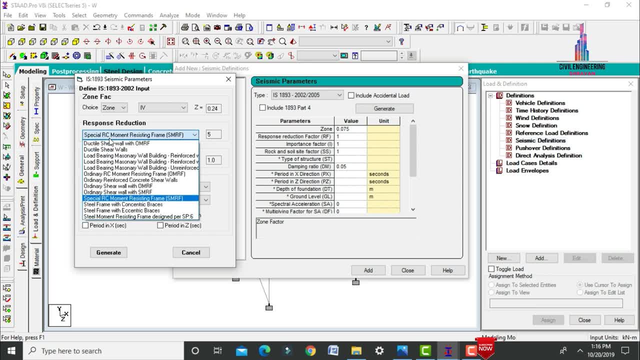 And we have to select this respected or special RC movement resisting frame. So after that we have to select the important factor for all general buildings And we have to consider the load conditions. So consider the structure type: is steel frame building with the soil medium condition? 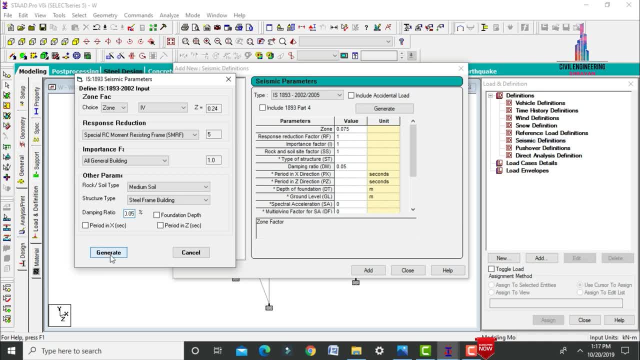 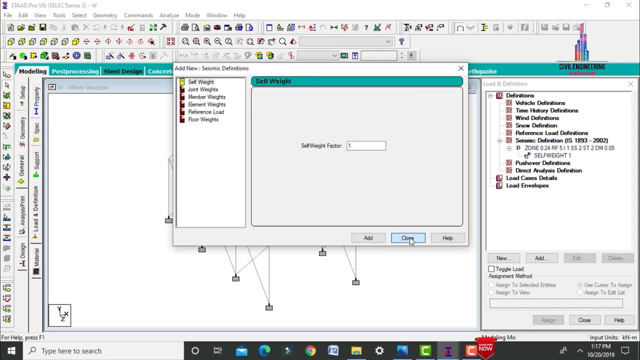 So here I am taking: damping ratio is 0.05, click on generate option So it will generate the parameters here. So after that, click on add button. So now we have to add the self-fit as well. add option, close option. 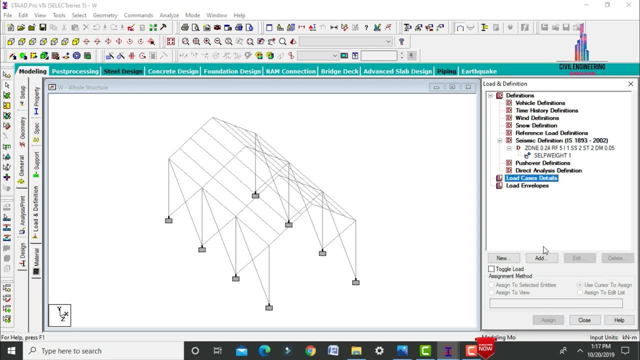 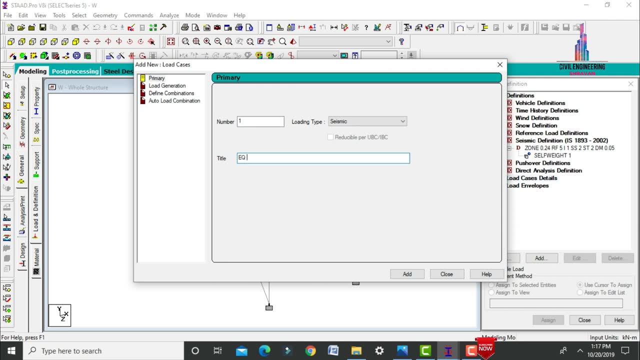 So after that we have to define the load case details. So select load case details option, click on add button. So initially we have to add the seismic loading condition. So here I am defining the earthquake load, which is in X direction. 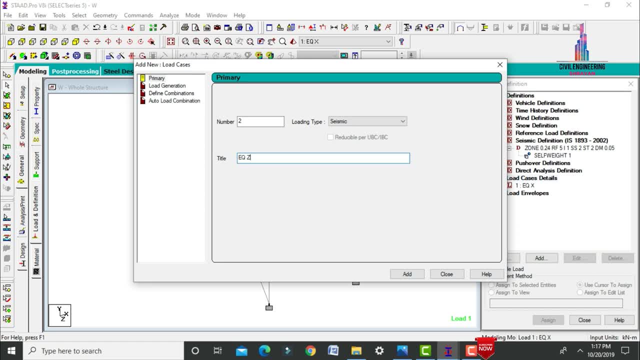 Again, I am selecting the earthquake load, which is in Z direction- condition add button. So after that we have to add the dead loading condition- DL add button. Again we have to add the live loading condition- LL- add it. 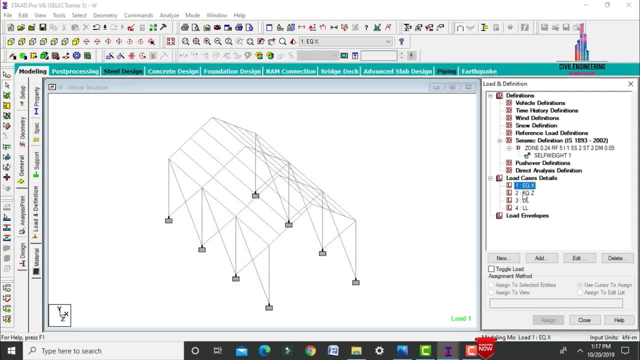 So after that click on close option. Now we have to select the earthquake load which is in X direction. condition We have to apply the forces which is related to the X direction only. So click on add button. So here we have to select the seismic load which is in X direction, with the factor as well. 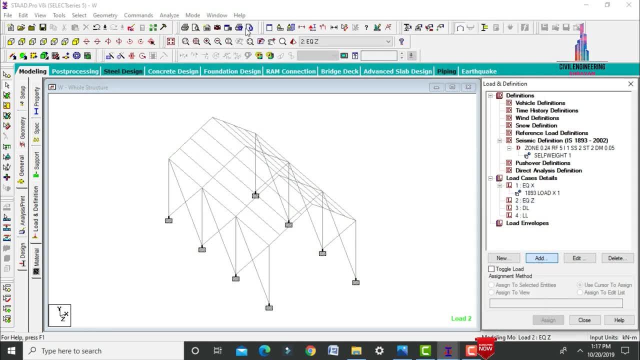 Add it- close option. Select earthquake load- Z- add button. In the same way, we have to select the seismic load, which is in Z direction with the factor 1, add button- close option. Now we have to select the self-fit for the dead loading condition. 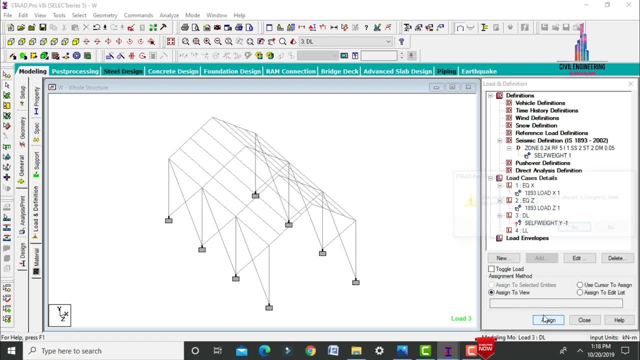 Click on add button. close option. Select the self-fit assign to view. assign yes option. So after that we have to select the live loading condition. So for this respective structure we have to apply the live load for the respective nodes. 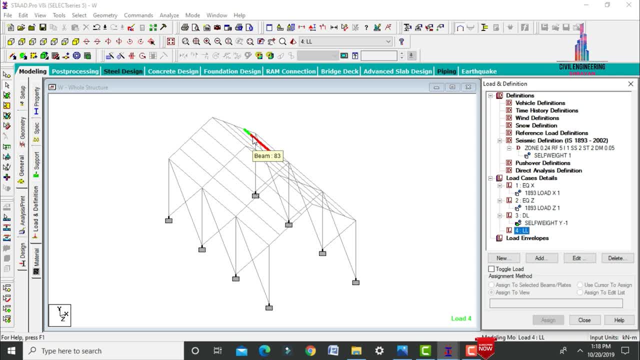 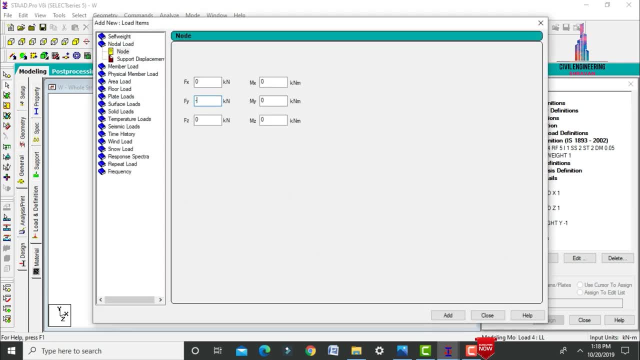 We have to apply the nodal load for these respective node cases. Okay, So click on add button. So here I am, selecting the nodal load which is having intensity of minus 20.. Just, I am assuming kilonewton which is acting for all the node cases. 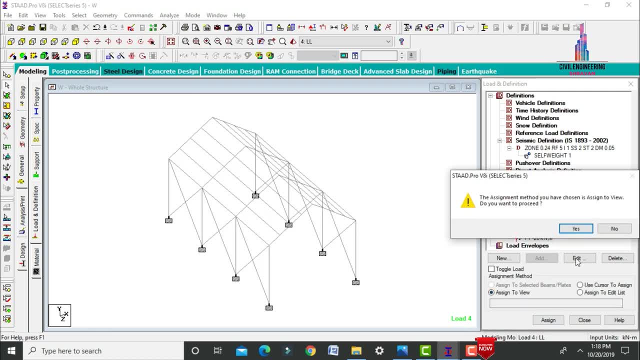 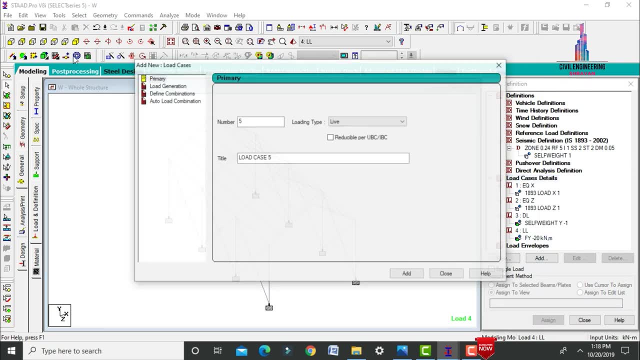 Click on add button. close option. Select the FY assign to view option. assign: yes. So after that we have to apply the load combinations. So select load case details, add button. So here we have to select the auto load combination generation as per the seismic load: dead load, live load. 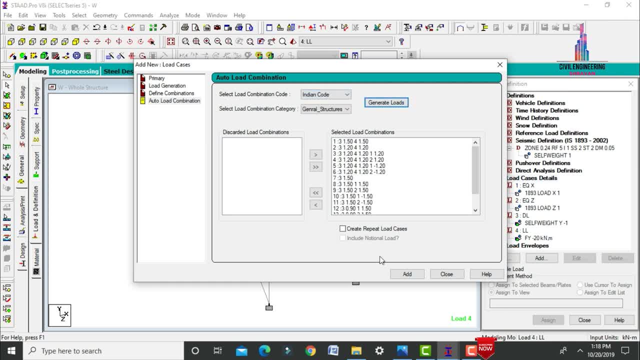 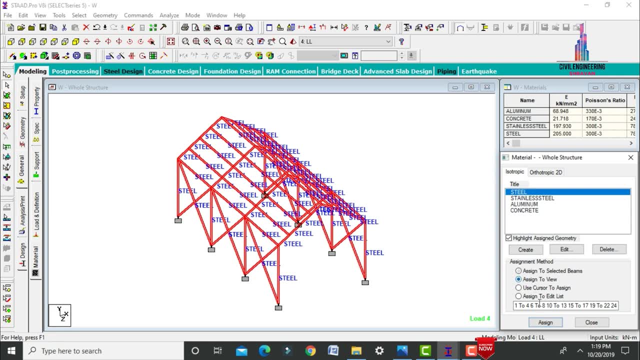 Select the load case code as Indian. Click on generate load combination. add button, close option. So after that we have to select the materials. Select the steel material. assign to view: assign: yes, So after that we have to analyze this respective model. 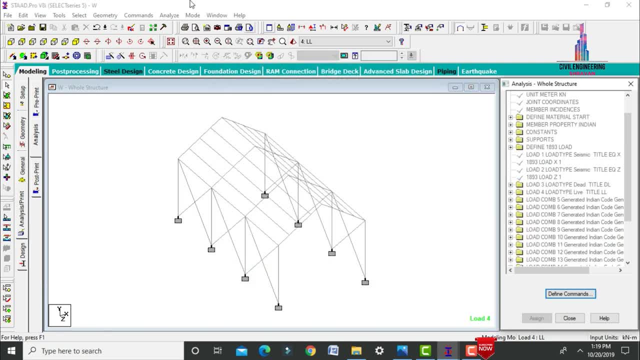 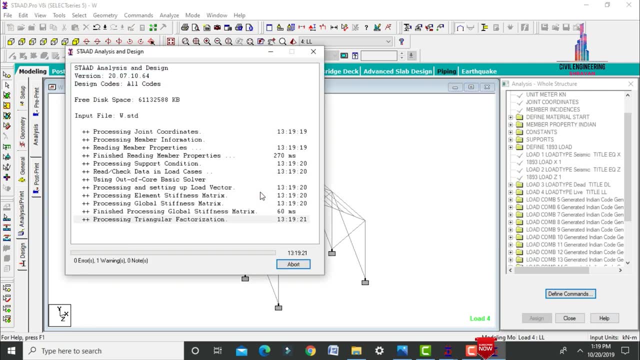 Go to analysis and print. hide your no print option. close option. Go to analyze option: run analysis, save it. So here we have to check the zero errors for this respective model. So here my model is checking for the zero errors. 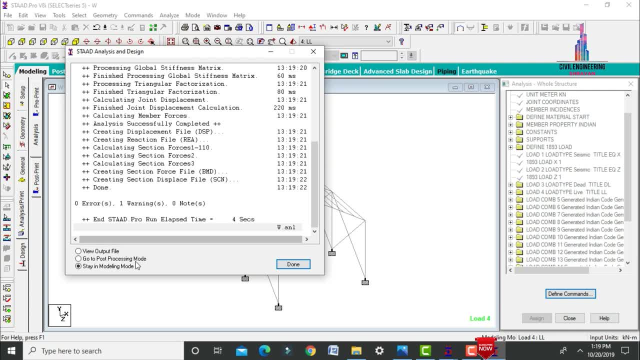 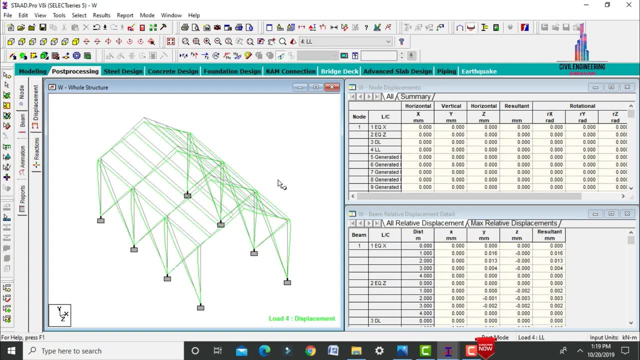 It was observed with zero errors. It was observed with zero errors here. Go to post processing mode option. click on done option. Click on apply. click on ok. So this is the deflection diagram for this respective model. Due to presence of the live loading condition, it was deflecting downward direction. 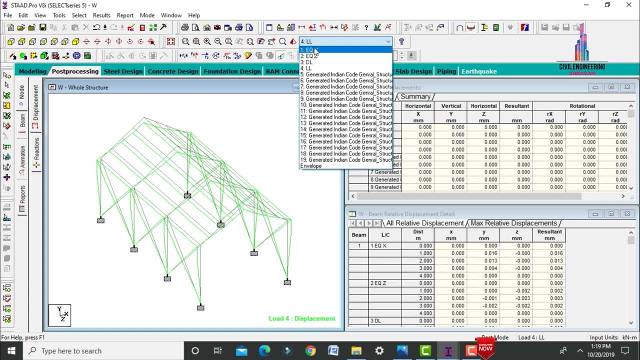 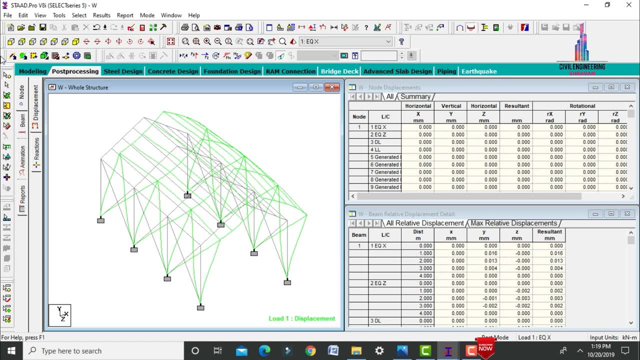 Why? Because we have applied the gravity load, which is in downward direction. So after that, select the earthquake load in x direction condition. Due to presence of the seismic zone 4, the building is deflecting in this respective x direction condition like this: 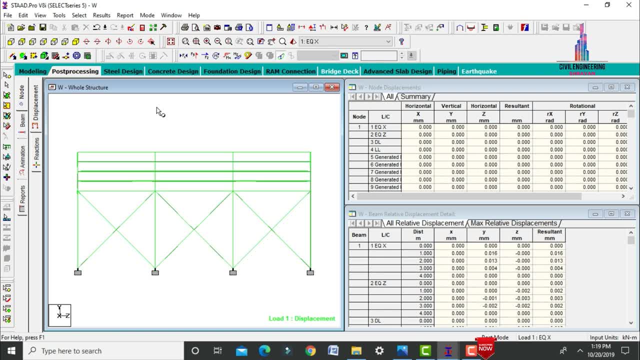 Ok, now we can see the deflection diagram Here like this. So after that select the side view, apply the load case as y direction load case. So this is the deflection due to presence of the seismic loading condition which is in y direction. 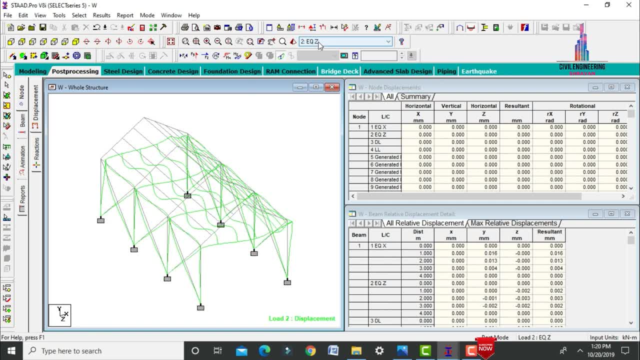 So after that we have to select this respective 3D view. So now we have to select the dead load condition or live load condition. This is the live load condition deflection diagram And this is the dead load condition deflection diagram. 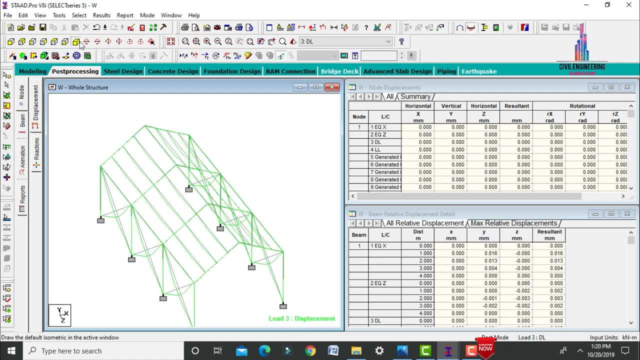 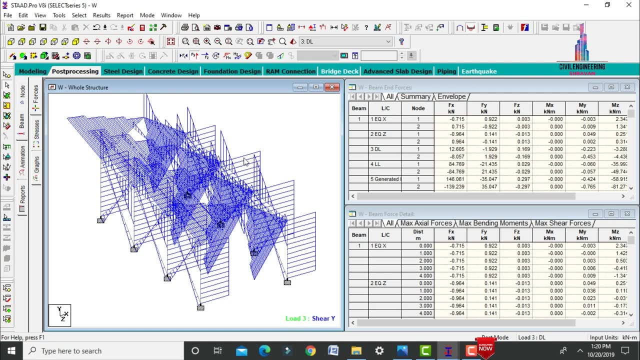 So after that we have to check the shear force diagram as well as bending moment diagram. So further select the beam here. Deselect the MZ, Select F5.. So this is the shear force diagram for this respective structure. So after that, select MZ value. 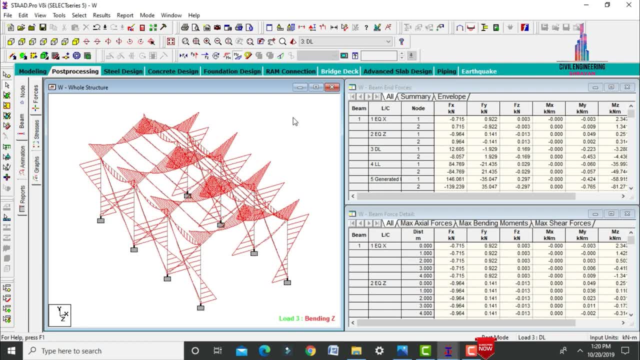 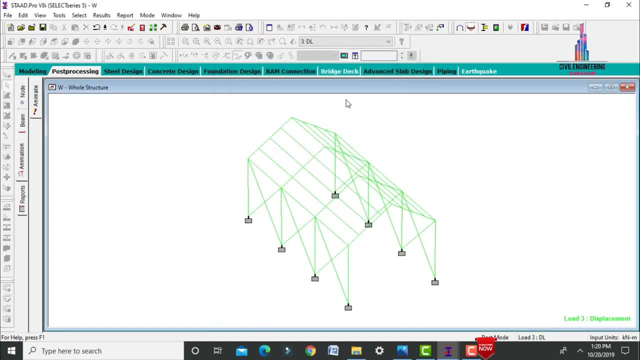 So this is the bending moment diagram for this respective structure. Ok, So after that we have to select the animation. Apply your deflection Apply. Ok, So this is the deflection diagram. due to presence of dead load. Due to presence of live load. 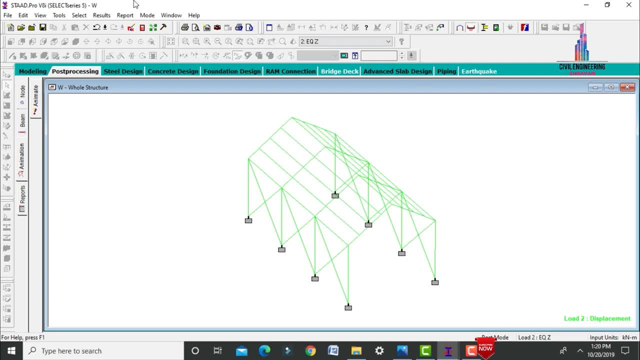 Again, due to presence of earthquake load in x direction, Earthquake load in z direction. So after analysis process is completed, We have to design this respective steel structure By using IS800 code. So further go to select the modeling option. 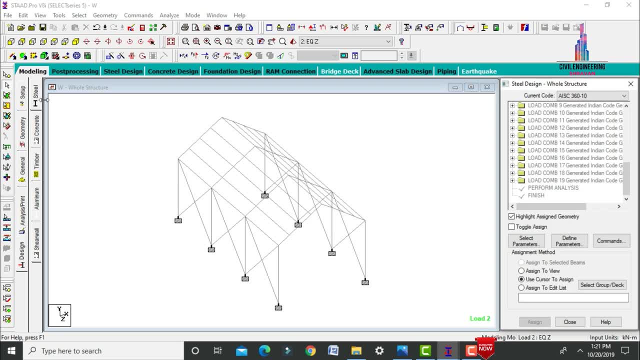 Click on design option. So here we have to select the steel design. So here we have to select the code as per IS800 LSD section. So it will be consisting of IS800 LSD 2007 here Select this. Click on select the parameters. 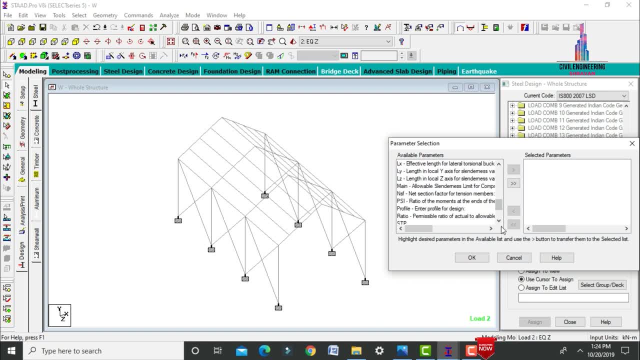 So here, initially, we have to deselect all parameters. From these parameters we need to pick only two parameters, which are related to the tracking parameter As well as yield strength of the steel. So select the track parameter initially. So after that we have to select the yield strength of the steel. 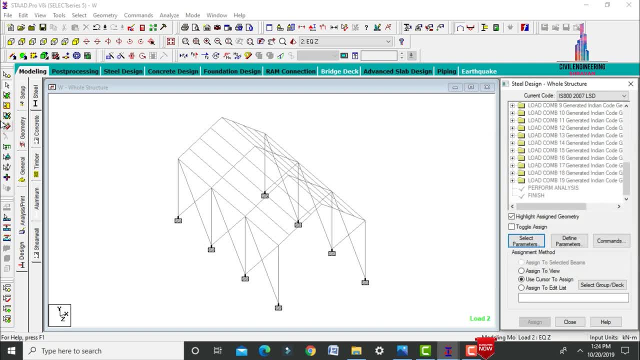 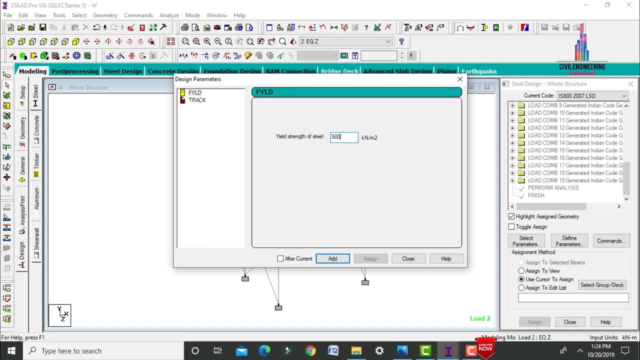 So here I am selecting yield strength of the steel. Click on ok. So after that, click on define parameters. Initially we have to define the yield strength value. So here I am assuming 500.. Fe 500 grade steel For this suspected steel members. 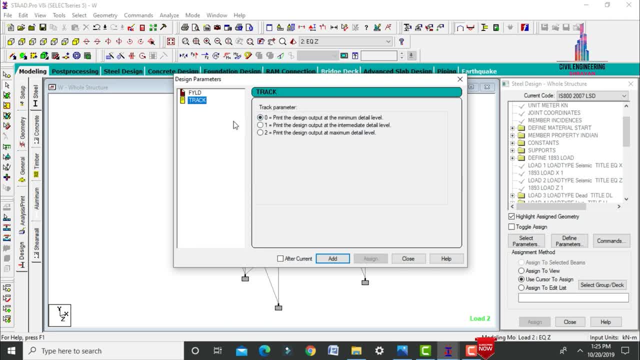 Click on add, So after that click on track parameter. It will be consisting of three values here: 0,, 1, 2.. 0 is nothing but Print the design output at the minimum detail level. 1 is nothing but print the design output at intermediate level. 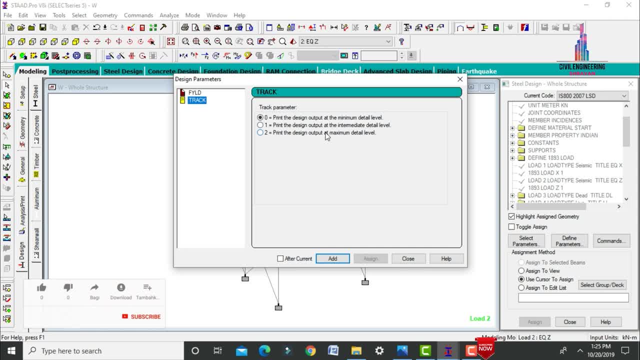 So second one is nothing but print the design output at maximum designing level. Ok, So from these respective parameters, just I am selecting as 2. Why? because we need to have the design data as per the maximum parameter level. So click on add button. 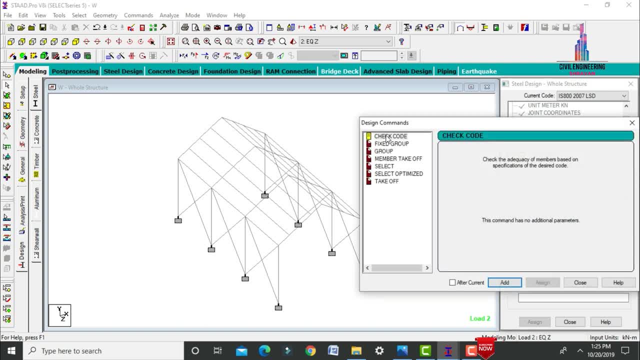 Close option. Select the comments option. So initially we have to select the check code option. So after that select the member take off. So after that select the select option- Add button. Select the take off option- Add button. 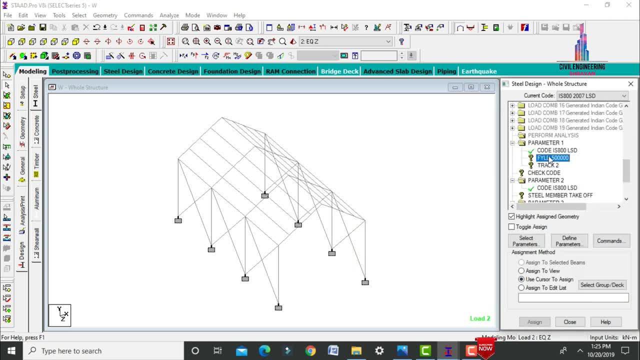 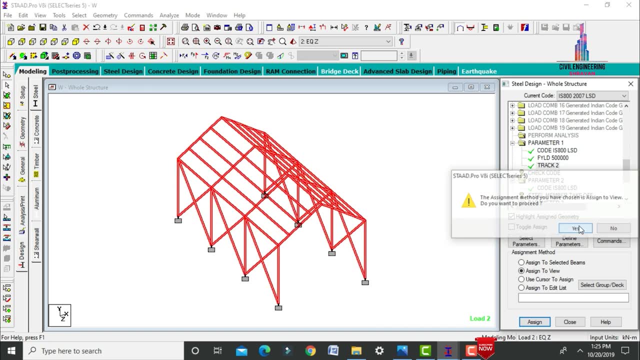 Close option. So after that we have to select the fy yield strength by using assign to view- Assign- yes option. Select track by using assign to view- Assign- yes option. Select the check code by using assign to view- Assign- yes option. 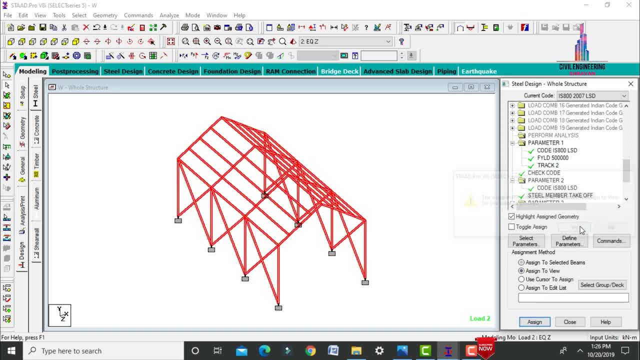 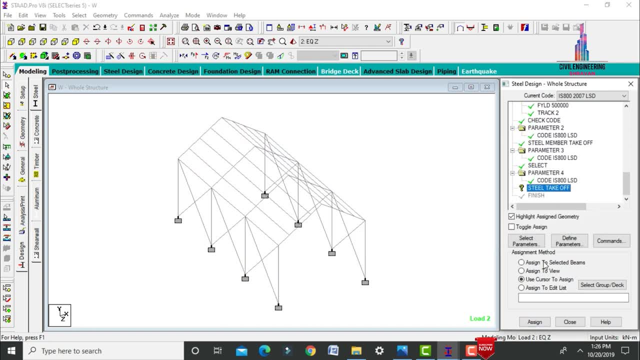 So select the steel member, take off Assign to view Assign: yes option. So after that we have to select the select option here again, Click on assign to view Assign: yes. Again, you have to select the steel, take off. Click on assign to view. 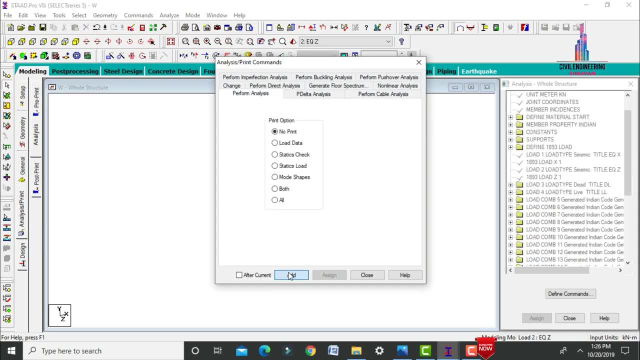 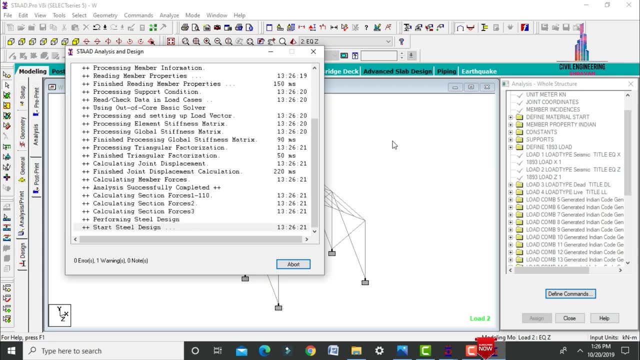 Assign yes. So after that go to analysis and print again. Add your no, print again Close option again. Go to analyze again, Run analysis again, Click on save option again. So again we have to check for the zero errors for this respective model also. 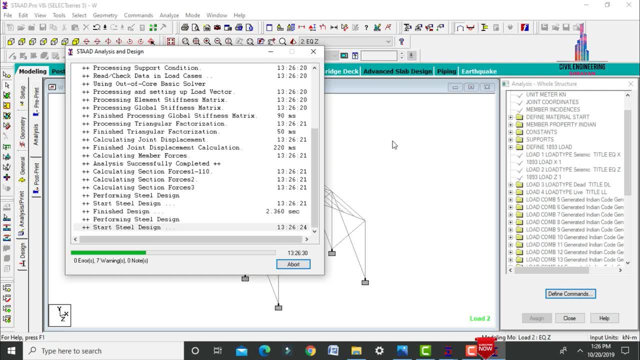 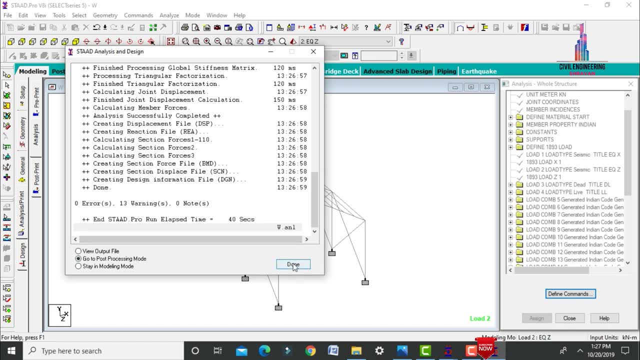 So here my model is checking for the zero errors. So here my model is observed with zero errors. Go to post processing mode again. Click on done option again Again select the beam, Deselect the bending event diagram. Select any one of that column. 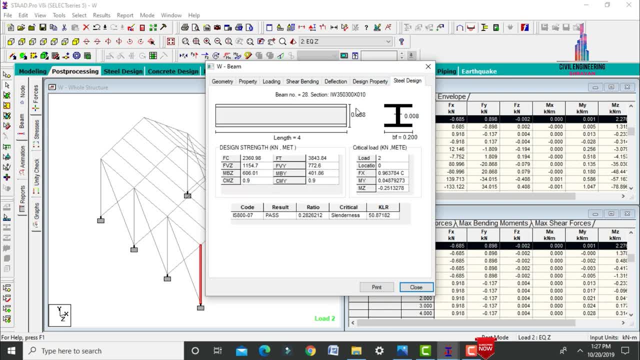 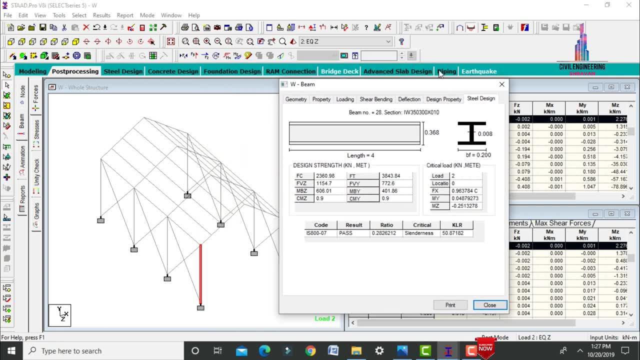 Double click on it. So this is the steel design results, which is consisting of DEBLU 350 cross, 300 cross, 10 mm section. So it is sufficient As per the definitions. we have assumed that, as per the safety, DEBLU 350 cross, 300 cross. 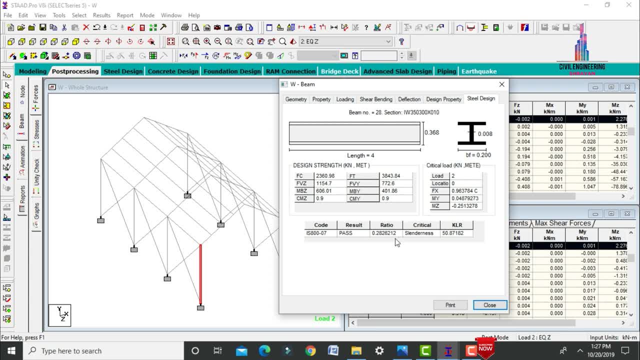 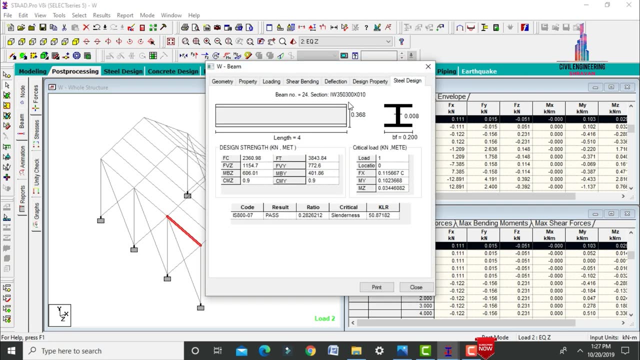 12 section. But as per the design results, as per the your consideration, it is showing that that steel, which is consisting of 350 cross, 300 cross, 10.. the sufficient for designing of this respected warehouse. again, i will select one more beam section. double click on it, click on steel design, so it will be consisting of same steel design. 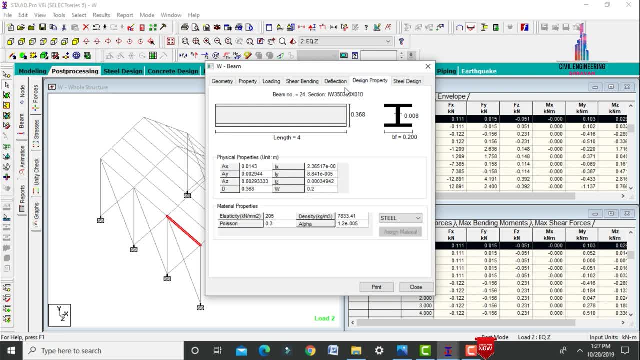 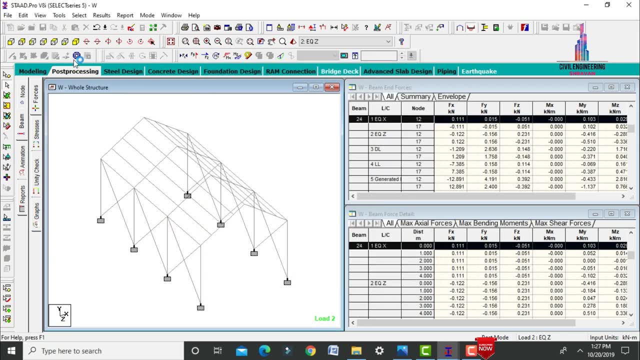 results, which is of 350 cross 300 cross 10. so this is the design property data deflection, shear bending loading. so after that we have to see the output file for this respected design. click on start output file option here. so click on results option here. so click on uh steel design. so it will. 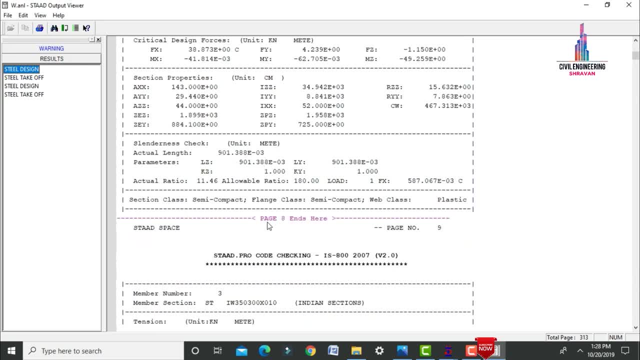 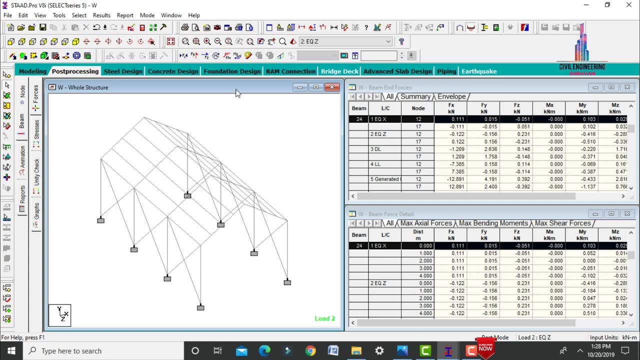 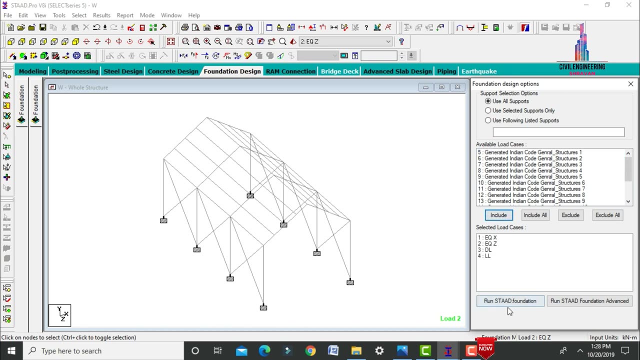 be consisting of each and individual calculation sheet for the respective steel members for this respected warehouse. okay, so after that we have to design the foundation for this respected warehouse, so select the foundation. so here we have to select the load cases which is related to earthquake load, as well as dead load, include: click on run start foundation. the fixed supports of this. 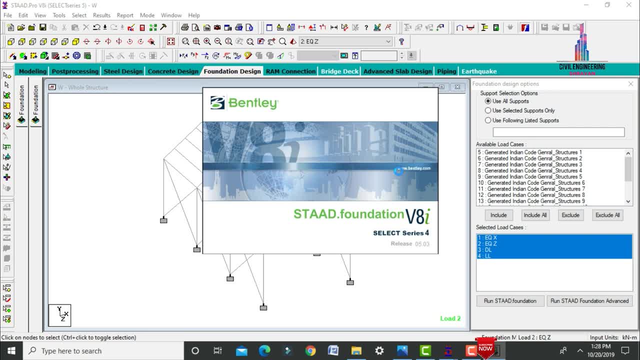 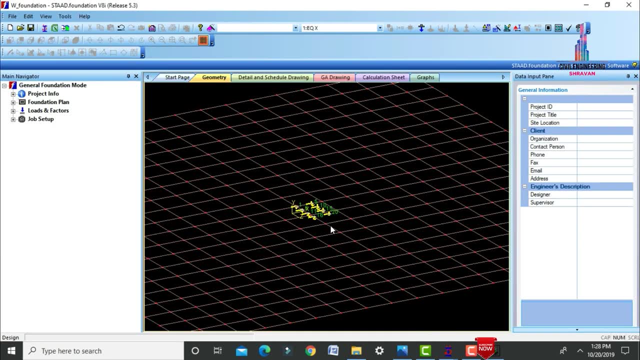 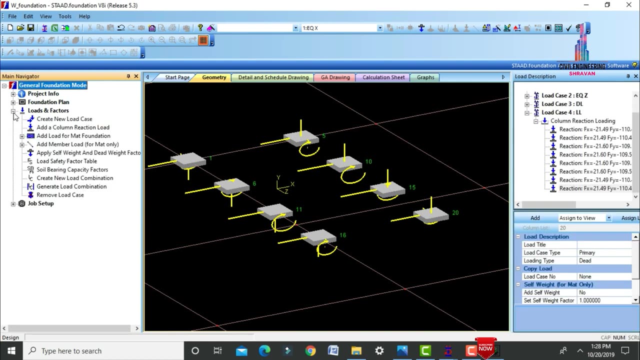 respected uh warehouse will be directly imported to the start foundation software. so these are the fixed supports we need to design the foundation for this respected fixed supports. before that we have to uh apply the load combinations. so select the loads and factors. so click on uh generate load combinations, so select. 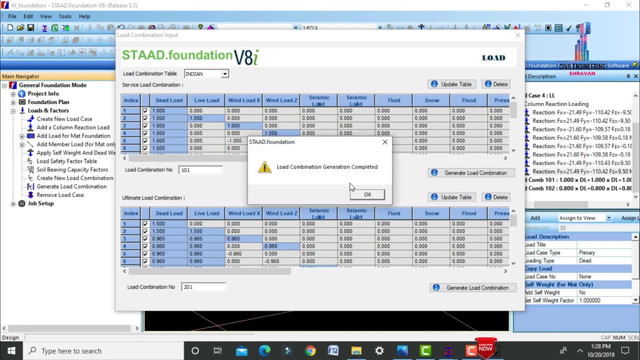 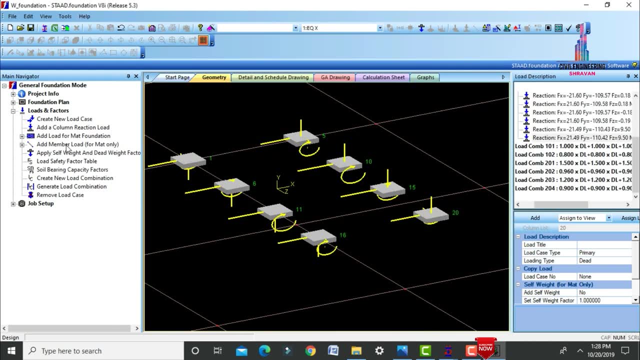 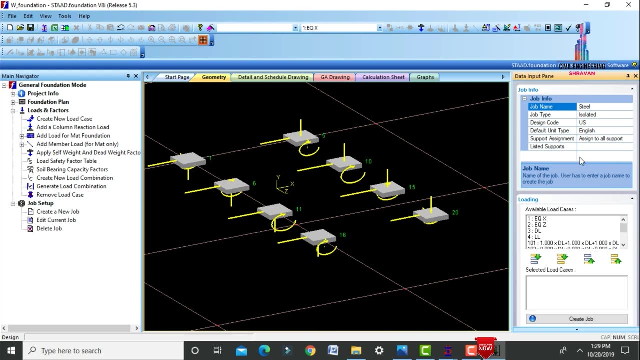 the indian standard system. click on generate load combinations as per the service load combinations. again click on generate load combinations and for the ultimate load combination, click on ok. now click on job setup. create job. so here i'm selecting name as steel. so select your isolator job type: isolated footing. so here i'm selecting indian and the units will be in assay system. 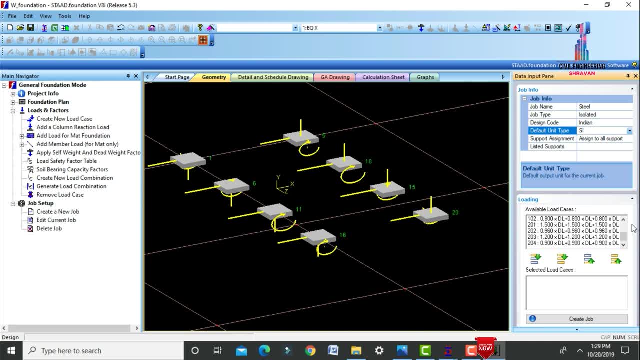 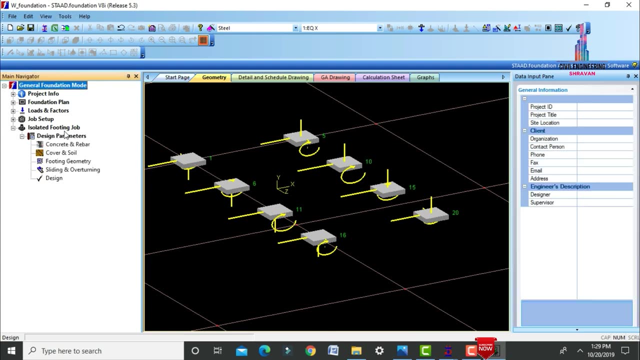 again you have to select the generated load combinations which is related to your respected 101, 102, 201, 202, 203, 204. include. click on create job so it will design this respected uh, isolated footing on the left hand side section here like this: so here we have to select the design parameter.